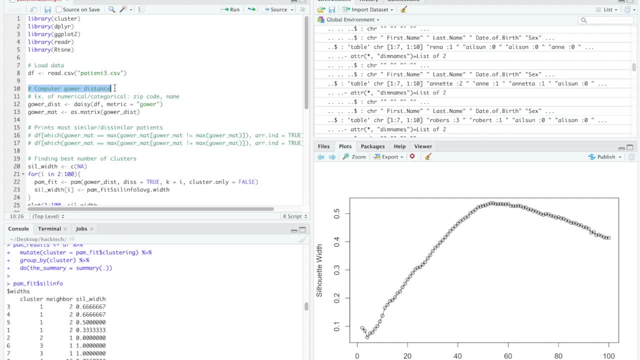 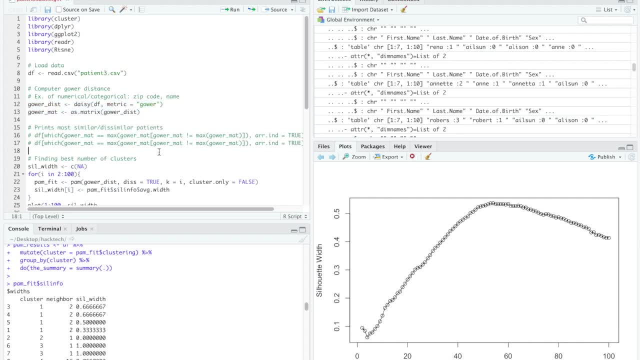 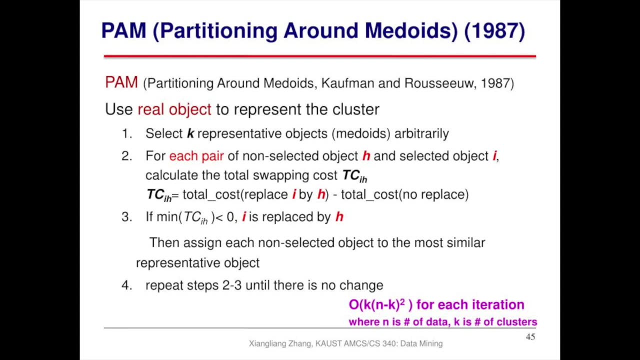 across individuals. The data set is then used to measure similarity across individuals. The calculated Gower distance fits well with the k-medioids algorithm PAM that we use a classical partitioning technique of clustering that clusters the data set of n objects into. 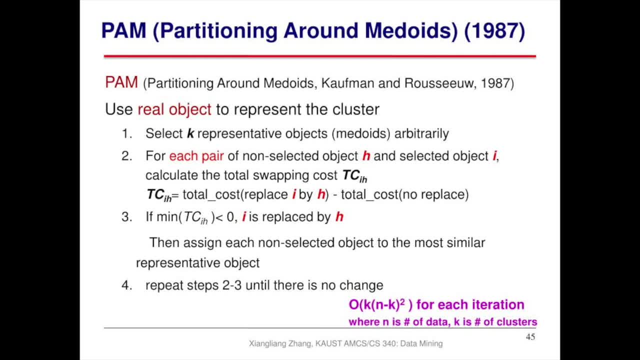 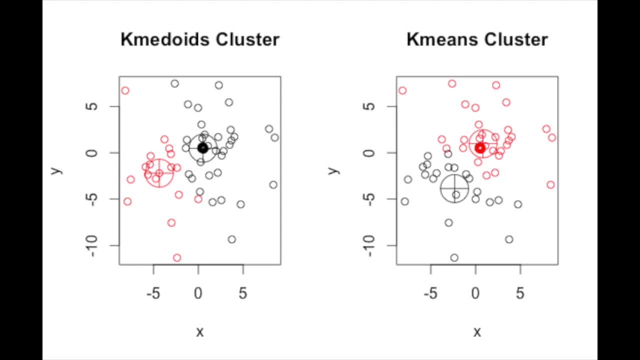 k clusters, known as priori. This unsupervised learning algorithm is similar to the k-means algorithm, but it is much more intuitive, much more robust to noise and outliers compared to k-means and, furthermore, produces a typical individual for each cluster, which is very 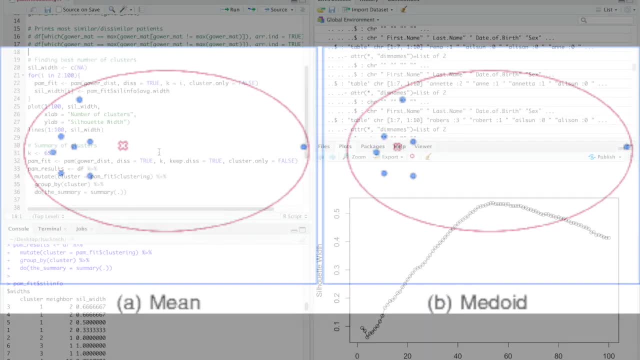 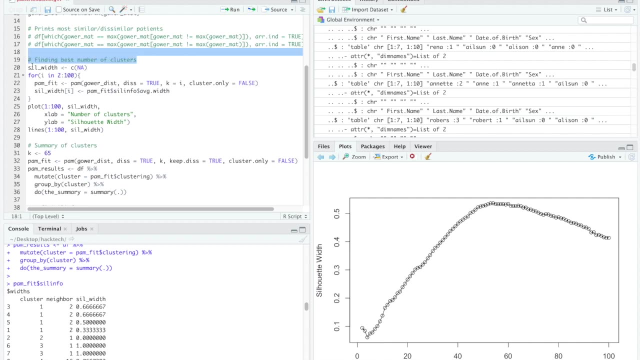 useful for interpretation. In order to make our algorithm more applicable to general data sets, we calculate for the silhouette coefficient in our next step, to determine the optimal number of clusters for PAM. The silhouette coefficient contrasts the average distance to elements in the same cluster with the average distance to elements. 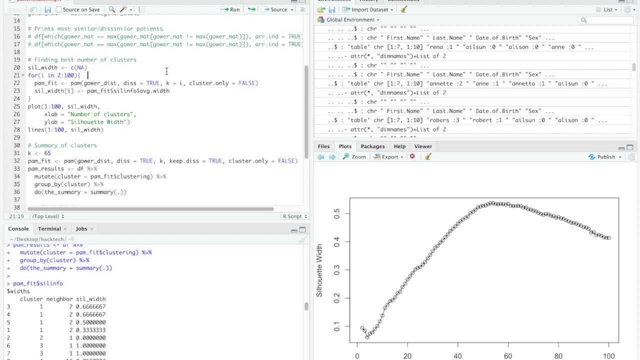 in other clusters, Objects with a high silhouette value are considered well-clustered. Just as an example, we find the optimal value from a range of 1 to 100 clusters and we can see from the graph that for the patient data set, the optimal number of clusters is close to. 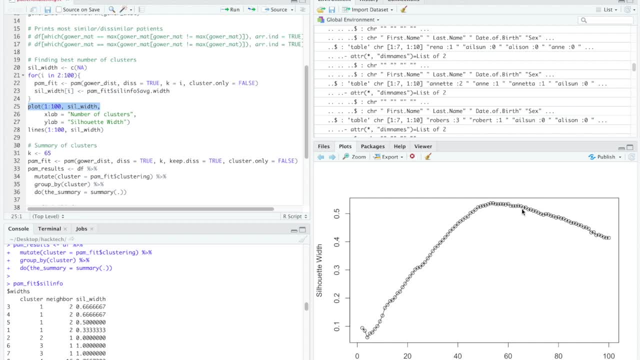 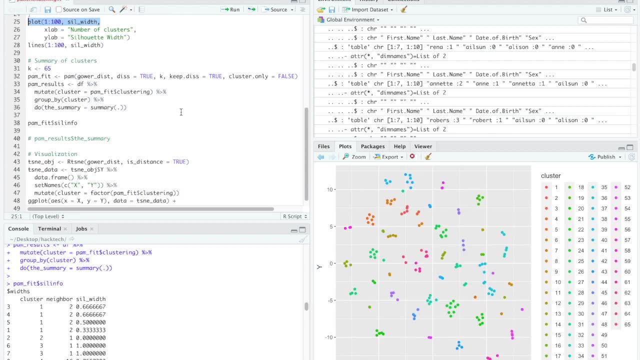 65, which is the actual number of groupings. Finally, we compute the 65 clusters with the dissimilarity matrix calculated by the Gower distance using PAM. A summary of the clusters can be produced using the summary function in R. that can be used for further data analysis in bigger data sets and we 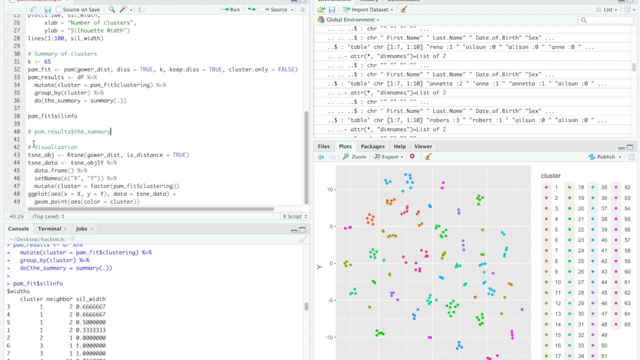 use T-SNE to produce a visualization of the clusters. SIL-INFO will display the observations, or, in our case, patients that are grouped together. From this we can compute the accuracy of our clusters, which was 95%. Real-world situations often deviate from ideal use cases that produce data sets with only 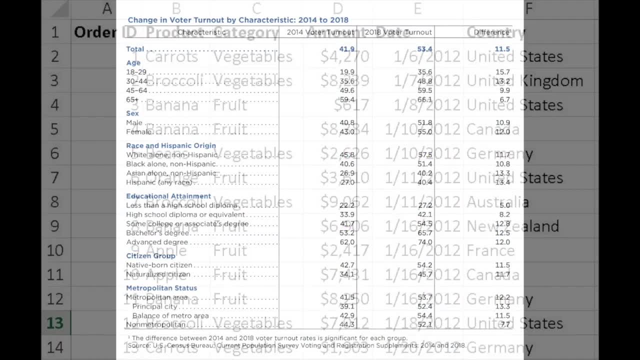 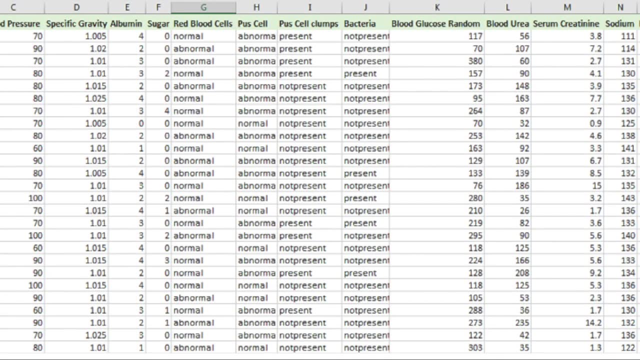 numerical features. Because of this, we wanted to develop this machine learning algorithm that would be able to analyze not just a patient data set, but any large data set with mixed-type data where numeric, categorical or ordinal features coexist.